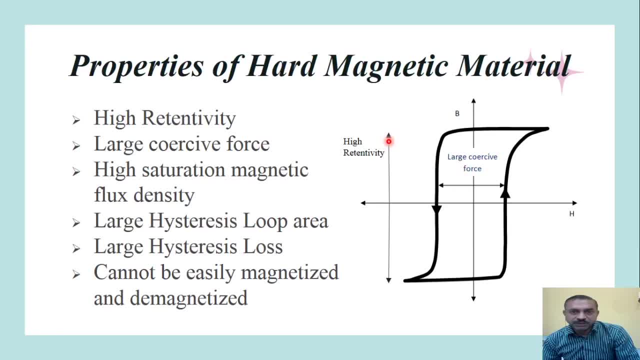 In this BH curve we can observe that these materials are having very high retentivity. It means that they will retain the high amount of magnetic flux within it once they get magnetized. Second is they have the large coercive force. 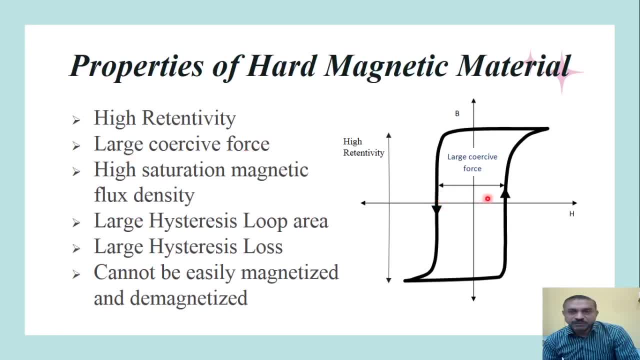 Coercive force is the force that is required to demagnetize the material completely. It means that they will have this high value of coercive force, that is ampere per meter, to make them demagnetized. Second third is the property that is here is the high saturation, magnetic flux density. 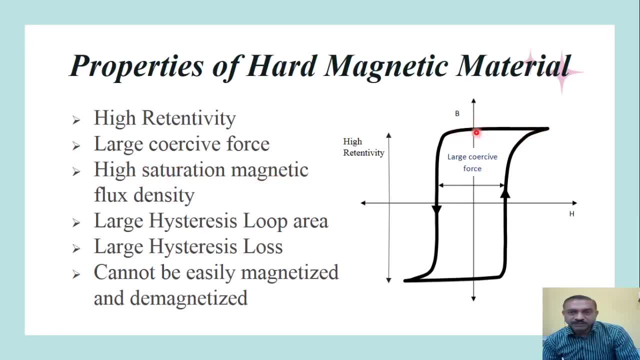 which we can observe from this graph that this material will have the higher level of magnetic flux density. Then we can see here is that this loop area of hysteresis is the large area and that is the requirement of hard magnetic material. 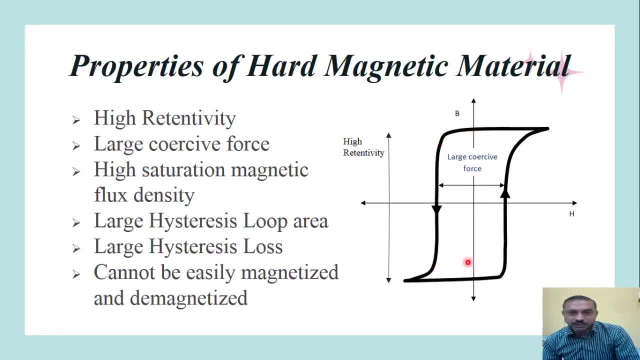 Because of this large loop area, we will have the large hysteresis loss that will take place in this material And this material cannot be easily magnetized and demagnetized. It means that once you magnetize this material, it will be difficult to demagnetize it. 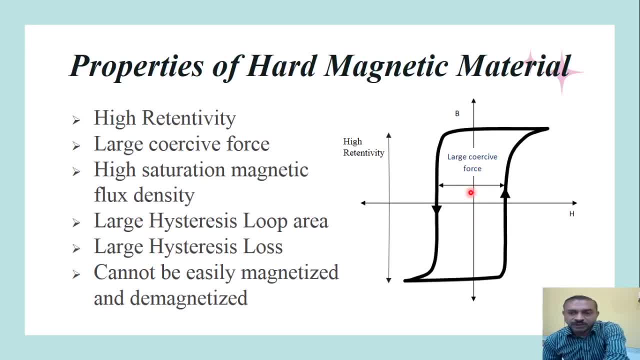 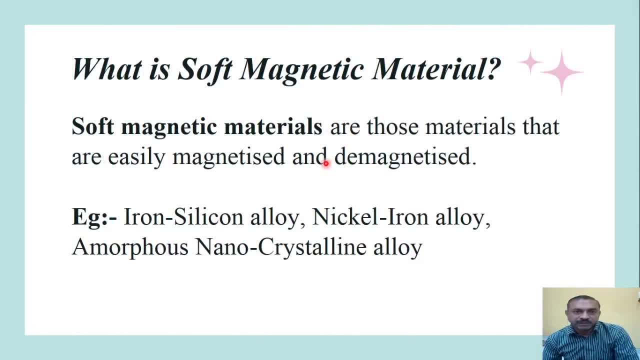 because we will be requiring very high or large value of coercive force to make them demagnetized. Now let us see what is the sub-magnetic material. Sub-magnetic material are those materials that are easily magnetized and demagnetized. 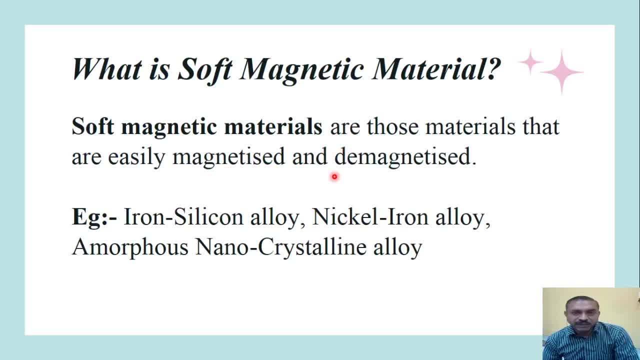 It means that we can make them magnetized and we can demagnetize as per our own requirement for a specific application. The most common material of this category are the iron-silicon alloy, the nickel-iron alloy, the amorphous nanocrystalline alloy. 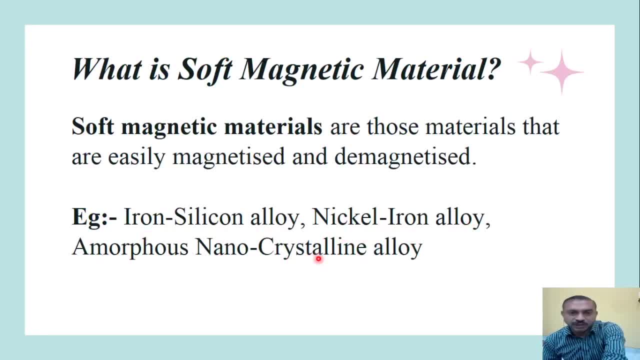 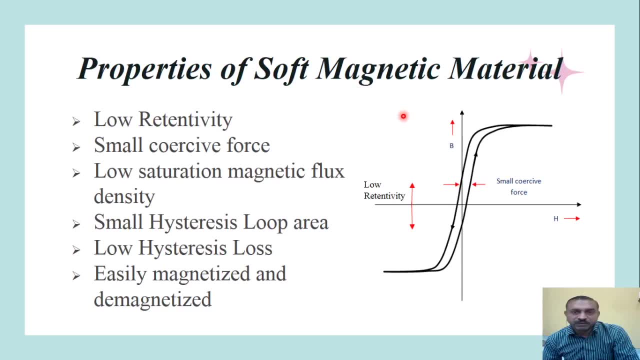 which is the most commonly used material in making the transformer in electrical power sector. Now let us see the properties of sub-magnetic material. To understand these properties again, we require to have the understanding of the BH curve and its look. 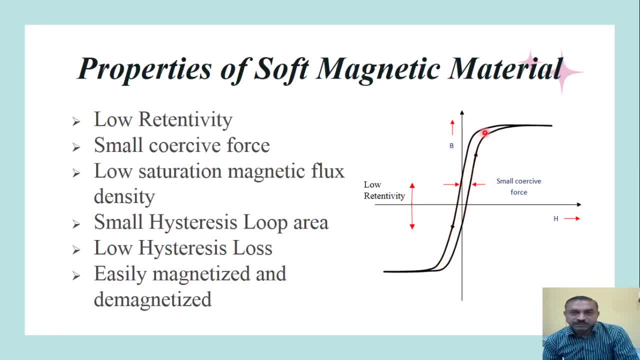 If you compare this BH curve with the previous, this is a BH curve which is having very thin cross-sectional area or very thin look. So if you observe from these points, you will get that there is low value of retentivity here. 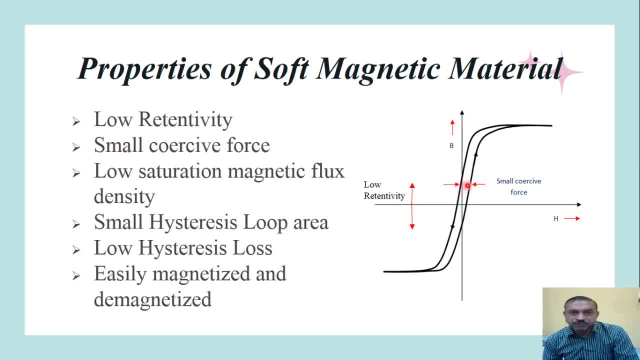 Then second is that here we require a very small coercive force to demagnetize the material. Then the magnetic saturation plug density is also of low value as compared to hard magnetic material. Then this area of the hysteresis loop is small. 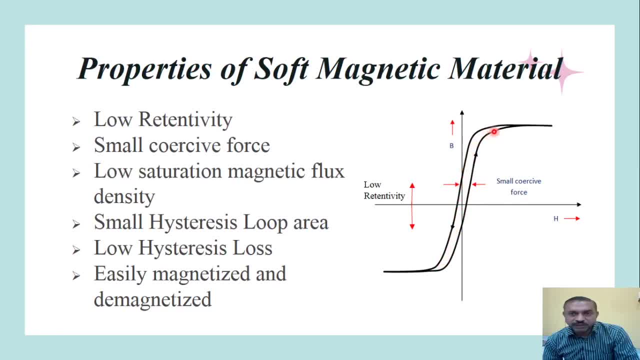 If area is small, then the hysteresis load that will take place in this kind of material will also be low or less. Then these materials are easily magnetized and demagnetized. So these are the key properties of sub-magnetic material. 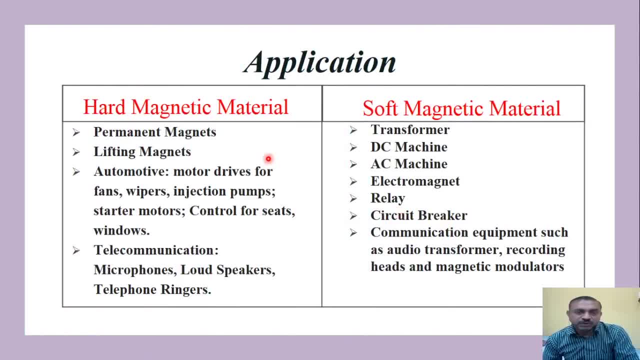 Let us see what are the applications of hard and sub-magnetic material. As we earlier discussed that the hard magnetic material are having large retentivity, large coercive force, higher saturation plug density, It means that they will be very suitable for making the permanent magnets. 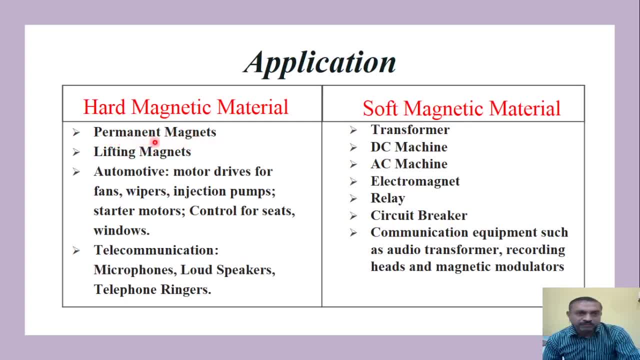 These magnets are to be used for longer period of time for their application, Then lifting magnets which are used to lift the certain type of goods material. Then they find a very wide application in automotive, That is for motor drives, for the fans, the wiper, the injection pumps, the starter motors, the control for seats and windows. 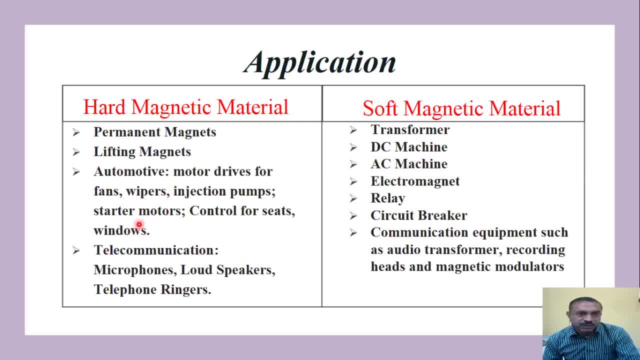 In any kind of the car, you will see this application of hard magnetic material. Then telecommunication is one of the field where we can find the application of the hard magnetic material in making the microphone, the loudspeaker, the telephone ringers. Now let us see. 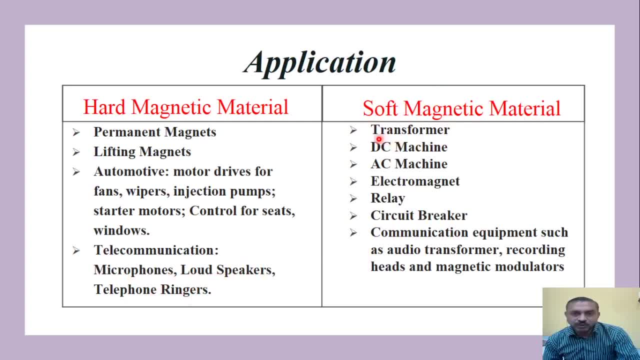 the application of sub-magnetic material. Sub-magnetic material are the most common and favored material for making the cores of the various electrical equipment or machines. The transformer core is made from amorphous materials. DC machine and AC machines they will have their core made from some active material. 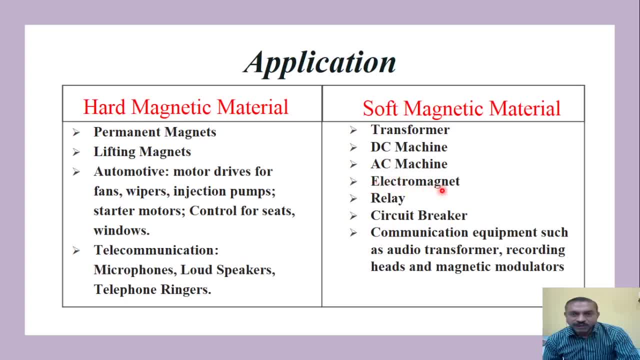 The electromagnet will be having their core as made from some magnetic material, That is, iron, silicon alloy. Then the relay will have have the use of some magnetic material for their operating function, then circuit breaker. then we can find application in communication equipment such as the rto transformer, recording aids and 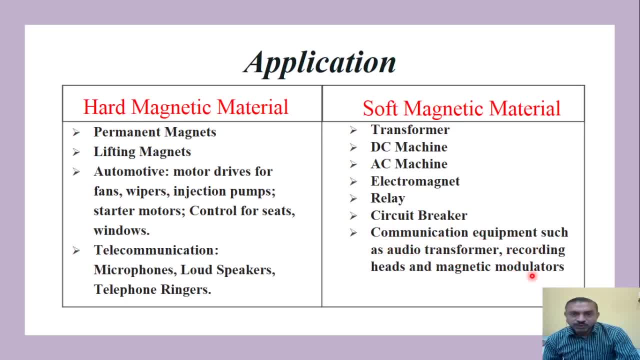 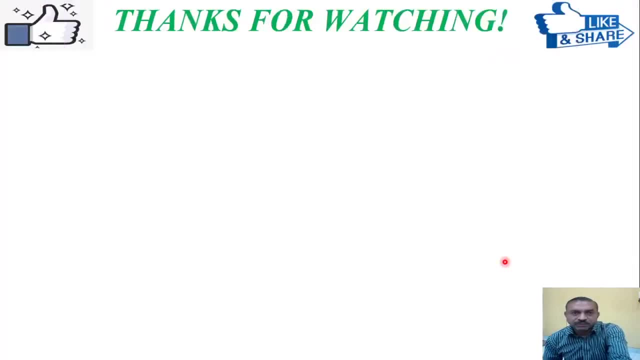 magnetic modulators. with these few important elements of understanding the soft and hard magnetic material, i am sure that you have got the basic idea and the knowledge of this hard and so magnetic material. with this and thanks for watching this video, do like the video and subscribe my channel. thank you. 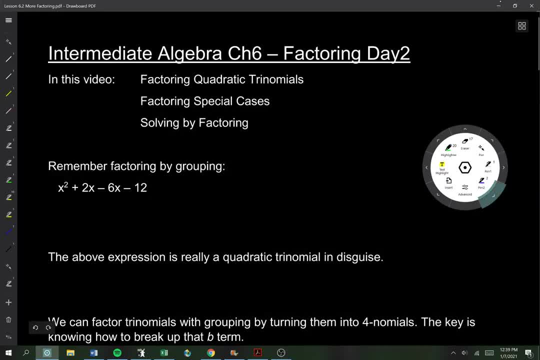 Let's talk some more today about factoring. We're going to be factoring quadratic trinomials, which we did a little bit in our last video. We'll do it by grouping, we'll do special cases, then we'll do some solving with it. So remember: factoring by grouping. Factoring by grouping is 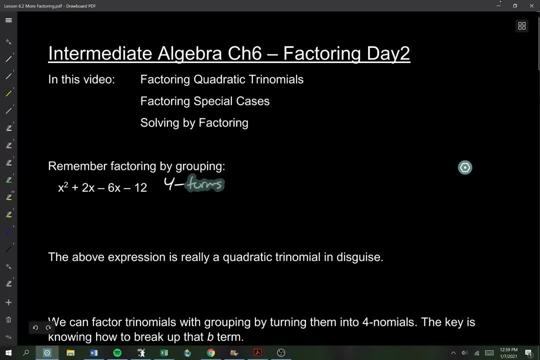 when you have four terms and you split those four terms into two groups and factor, pull the greatest common factor out of those. So I'm going to slash this in half right here and I'm very careful to keep this negative with that 6x over there. Out of the left half I can pull out an x. 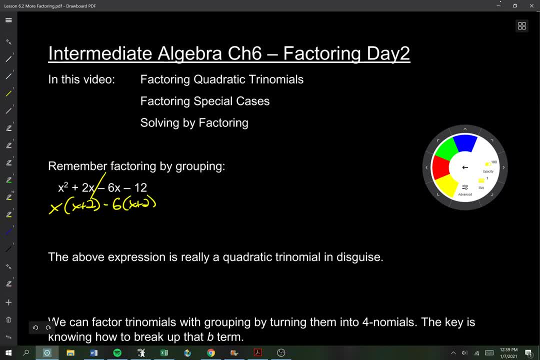 Out of the right half I can pull out a negative 6. And since these two factors are the same, these two things combine to be one factor, and x plus 2 is the other. So that's factoring by grouping. Now the thing is, this is really a quadratic trinomial, Trinomial. 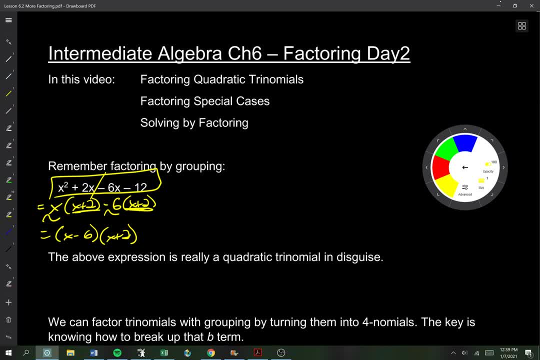 means three terms. It has four terms, but it's really a quadratic trinomial, because we could write it as x squared, x squared minus 4x minus 12. We could combine these two. So what this tells us is that we can. 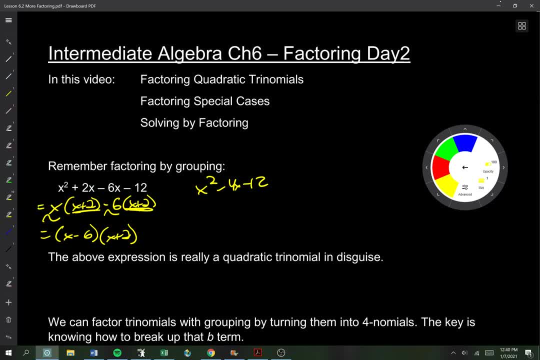 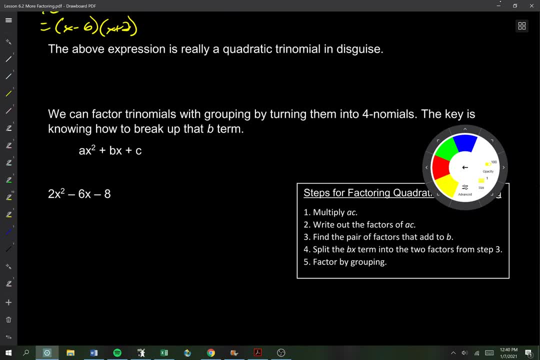 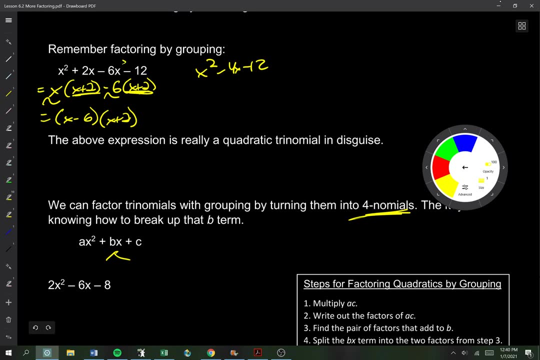 factor trinomials if we can make them into four termed expressions. So we're going to use factoring by grouping and turn a three termed expression into a four termed expression. The key is splitting up this b term right Like this, this b term negative 4x, was split into plus 2 and minus 6x.